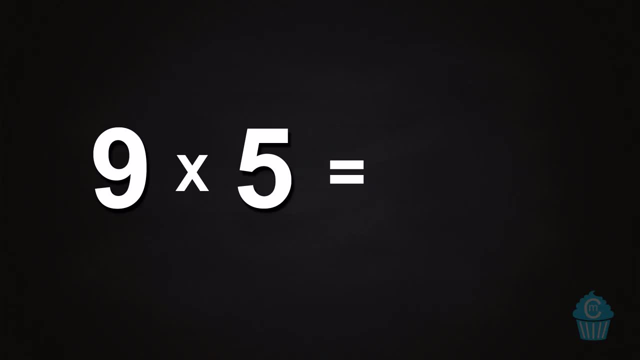 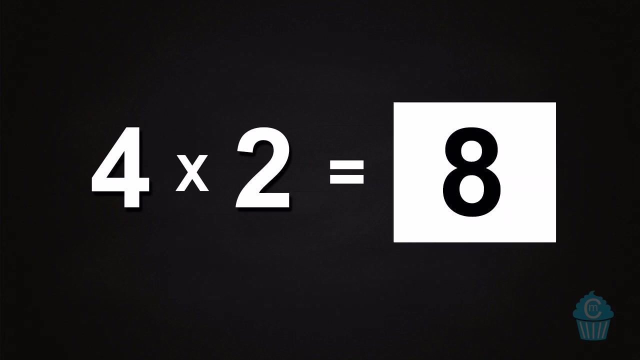 12. 9 times 5,, 45.. 3 times 4,, 12. 2 times 3,, 6.. 4 times 2,, 8.. 7 times 4,, 28.. 6 times 4,, 24.. 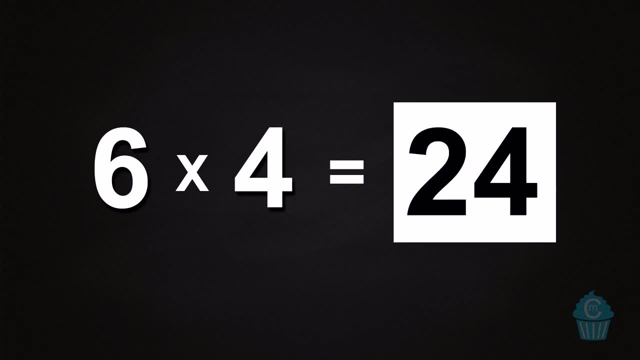 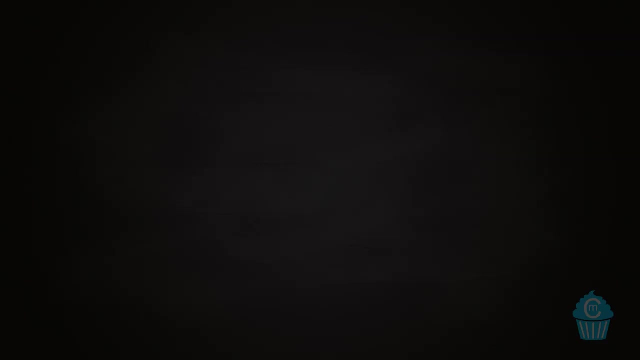 6 times 4, 24.. 6 times 8, 48.. 6 times 8, 48.. 6 times 8, 48.. 7 times 6, 42.. 7 times 6, 42.. 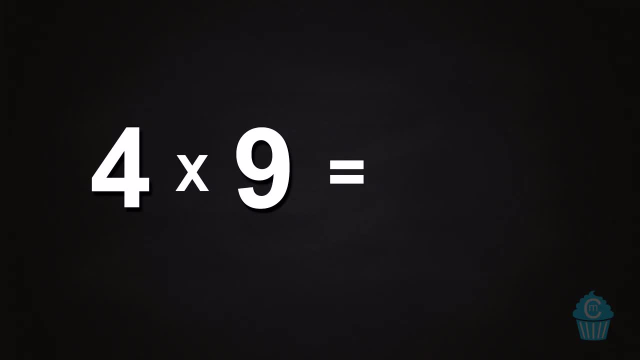 7 times 6, 42.. 4 times 9, 36.. 4 times 9, 36.. 4 times 9, 36.. 9 times 8, 72.. 9 times 8, 72.. 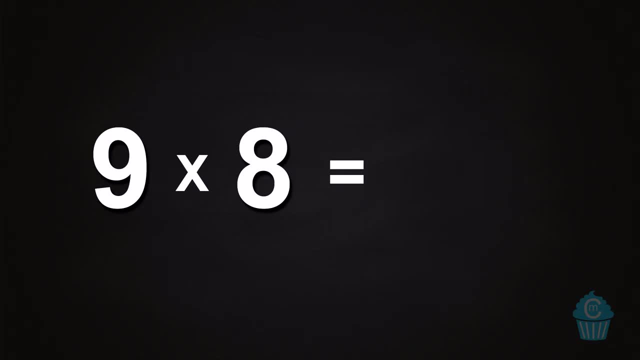 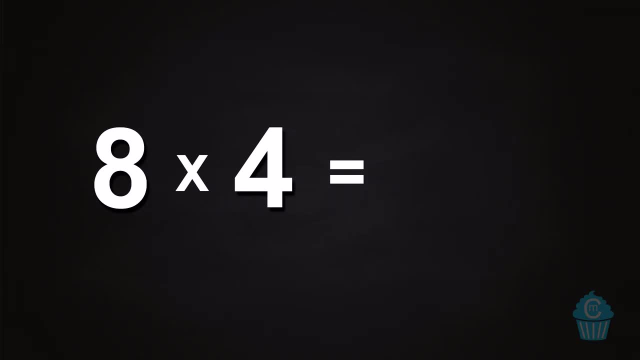 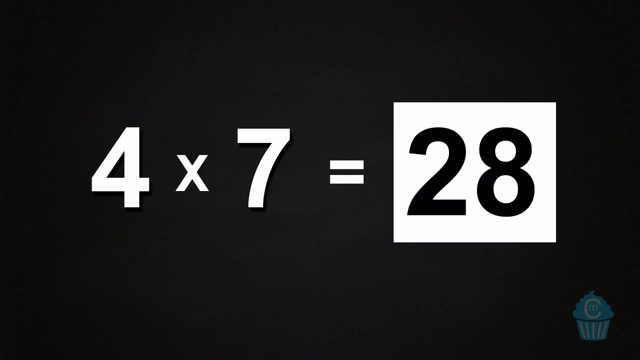 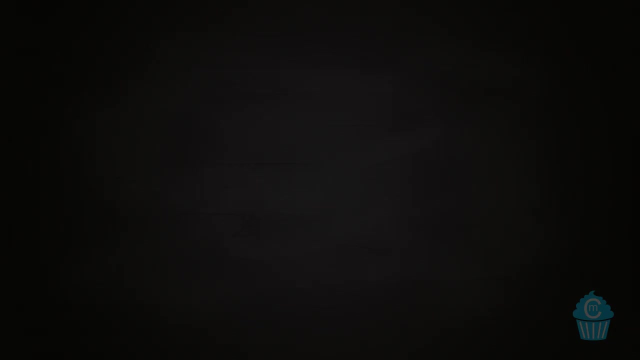 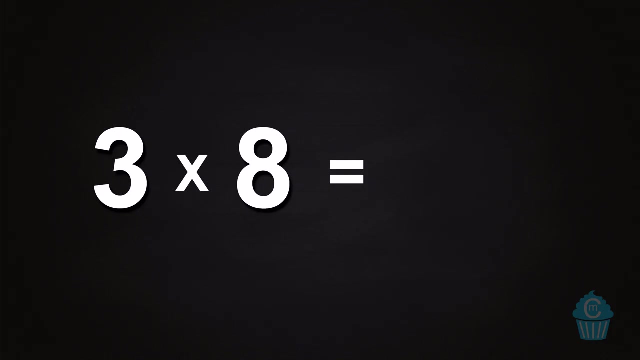 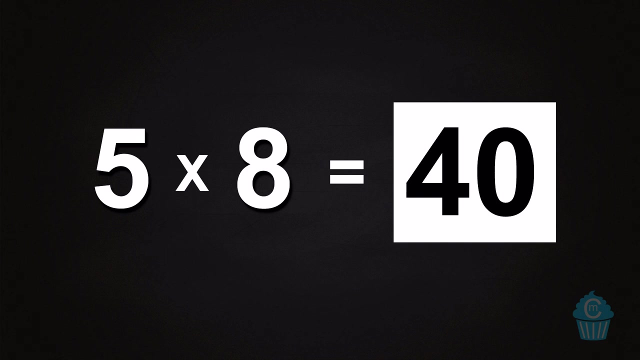 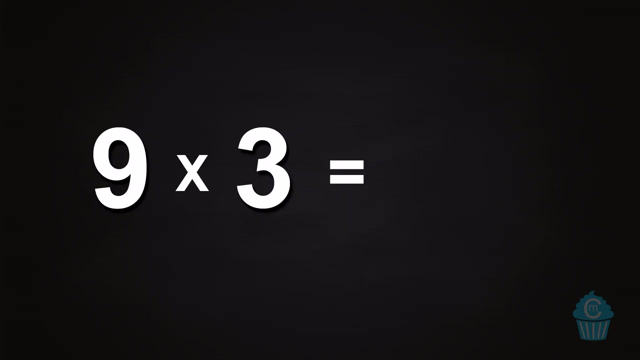 5 times 9,, 45.. 7 times 7,, 49.. 3 times 8,, 24.. 6 x 3, 18, 5 x 8, 40, 8 x 6, 48, 9 x 3, 27, 4 x 5, 20. 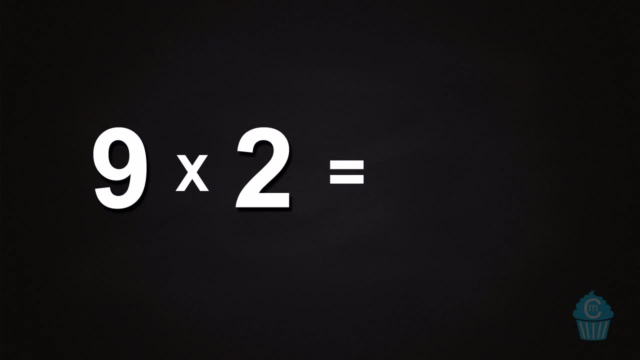 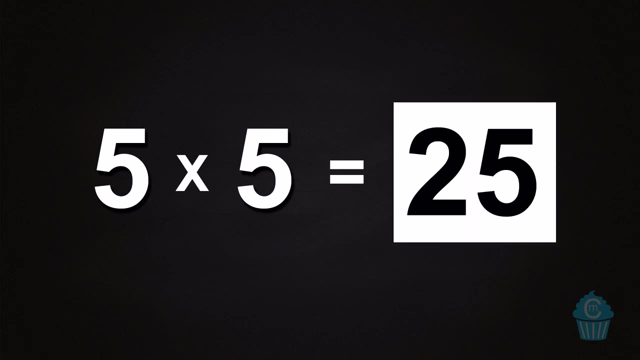 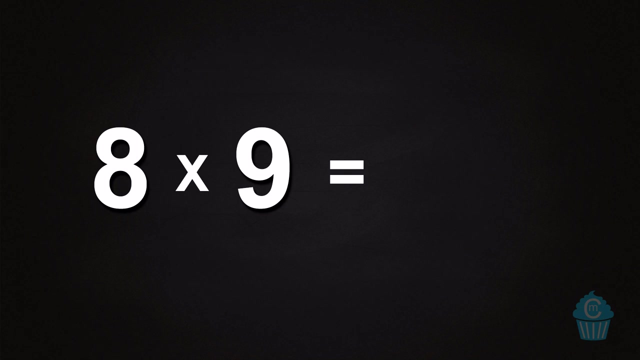 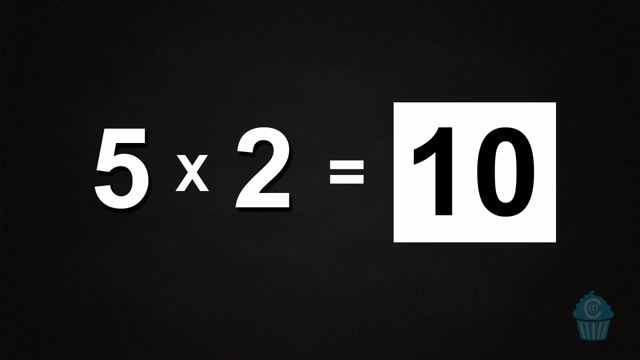 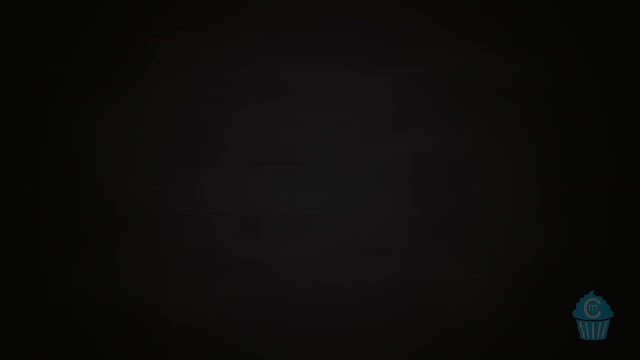 9 x 2, 18, 5 x 5, 25, 4 x, 4, 16, 8 x 9, 72, 7 x 3, 21, 5 x, 2, 7 x 8, 56, 3 x 3, 9. 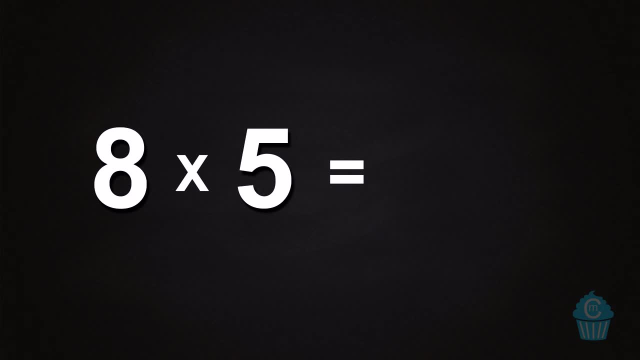 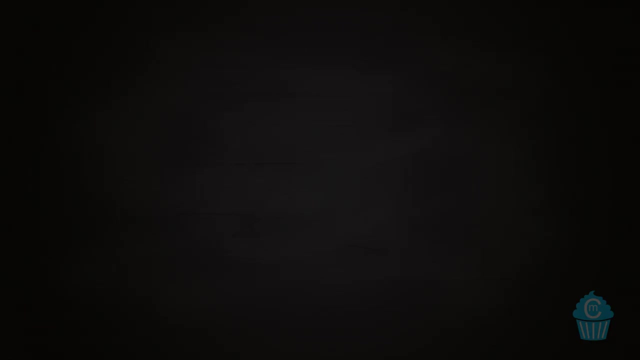 8 x 5, 40, 2 x 5, 10, 5 x 6, 30, 2 x 9,, 18, 6 x 5, 30, 3 x 9,, 27, 7 x 4, 28. 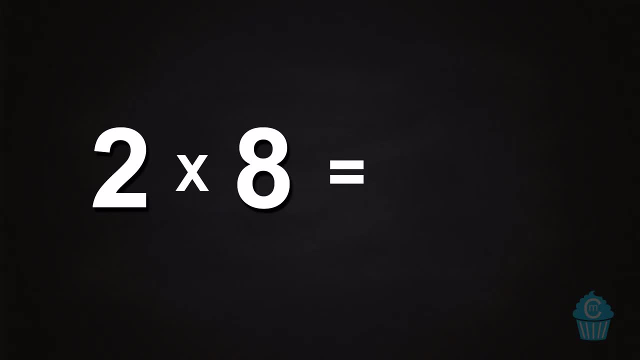 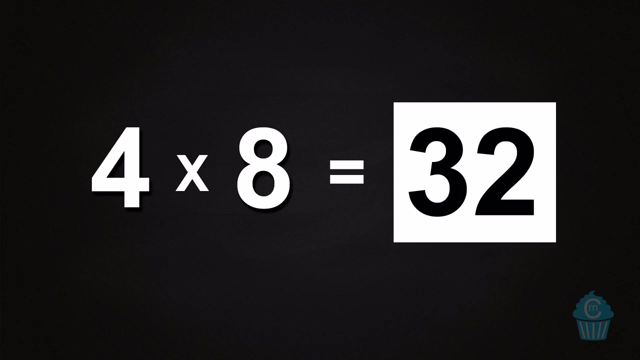 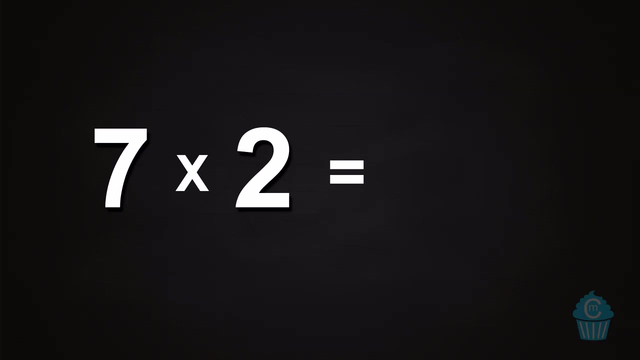 7 x 4, 28, 7 x 4, 28, 2 x 8, 16, 8 x 7, 56, 4 x 8, 32, 9 x 7, 63, 7 x 2, 14. 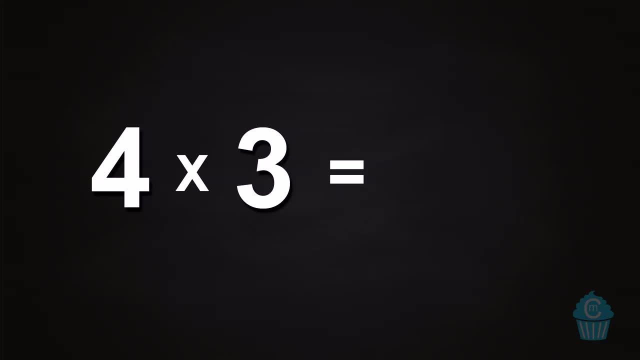 4 x 3,, 14, 4 x 3, 14, 4 x 3,, 14,, 12, 4 x 3,, 14,, 12, 4 x 3,, 14,, 12, 7 x 9, 63. 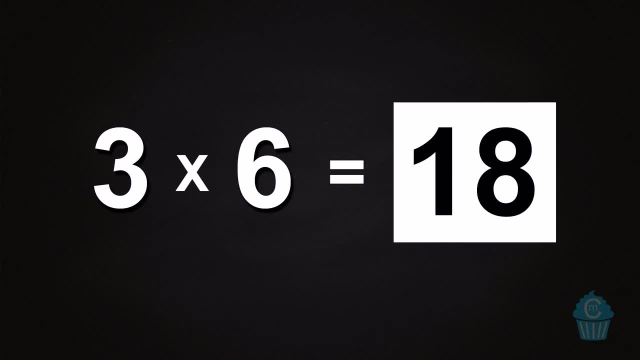 7 x 9, 63, 3 x 6, 18.